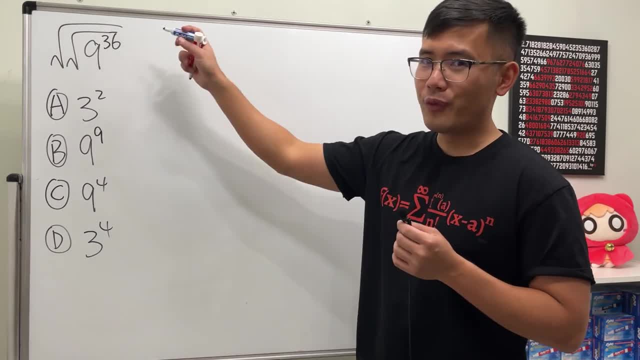 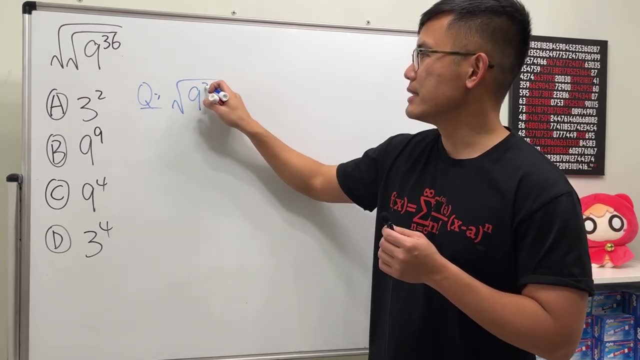 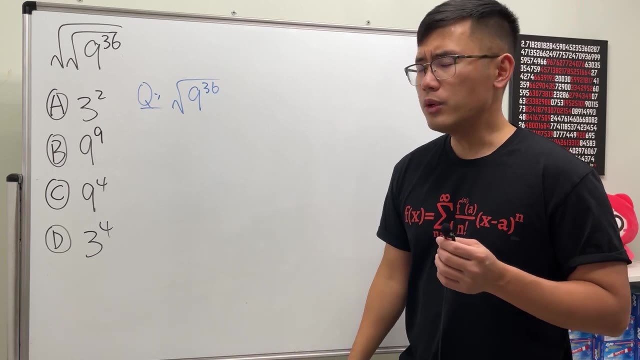 first Done. Okay, Before I go for this question, let me just go over the concept for you guys first. So let's just take a look at square root of 9 to the 36th power. This is pretty interesting because 9 and 36, they are both perfect squares. So can we just go ahead and do the square root of? 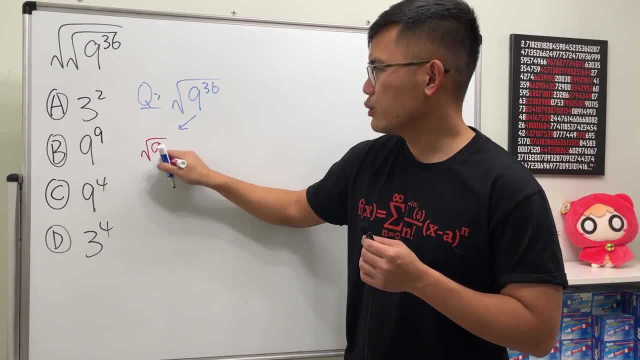 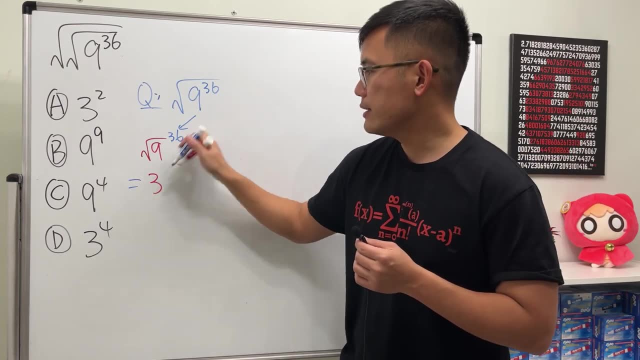 9 first. In that case, we are looking at square root of 9 for the base and then just keep the power to be the same. In this case, we will end up 3 raised to the 36th power, Or should we just? 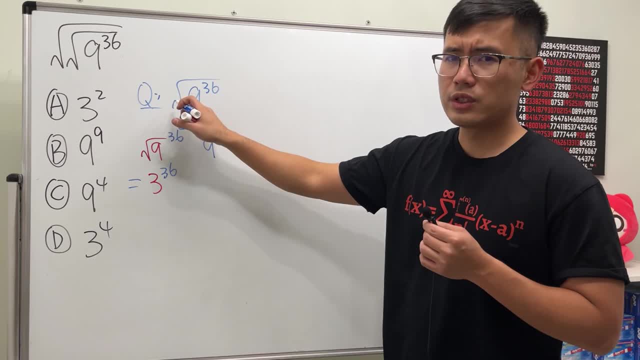 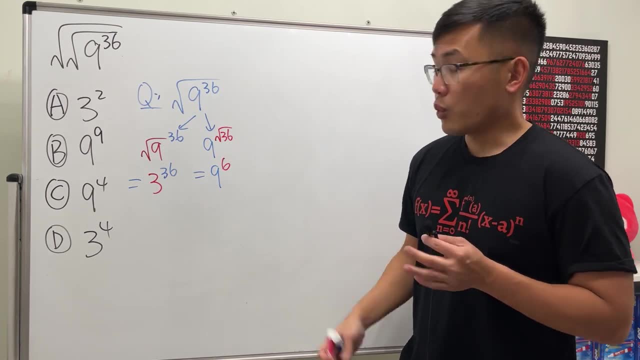 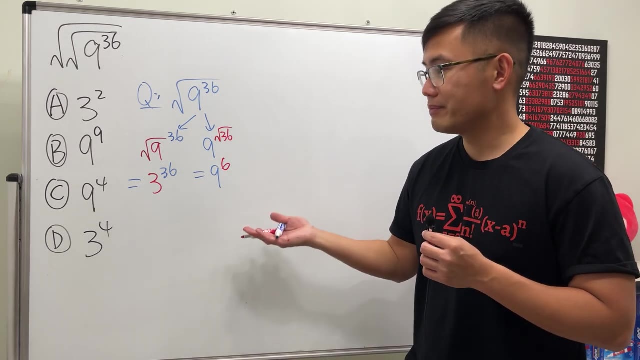 keep the base as 9 and then we do the square root of 36.. In that case we get 9 to the 6th power. So what do you guys think? Which one is correct? Or maybe both, Or maybe neither? The answer is: 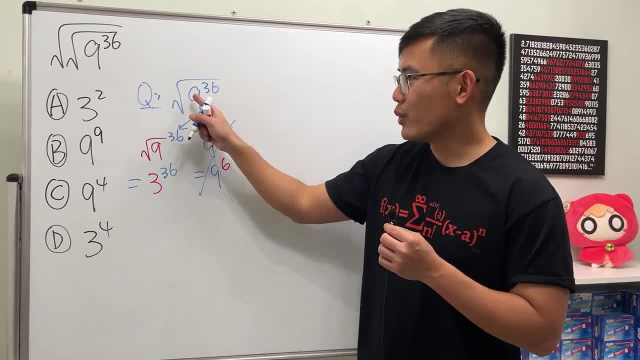 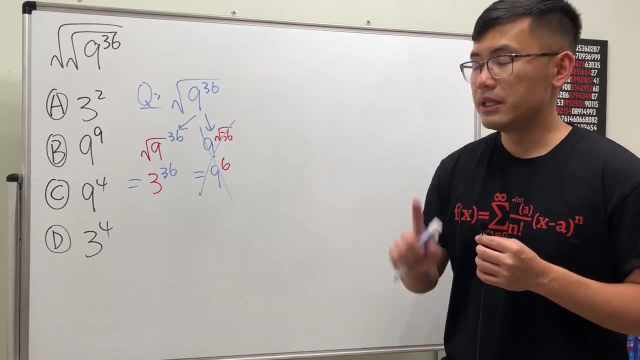 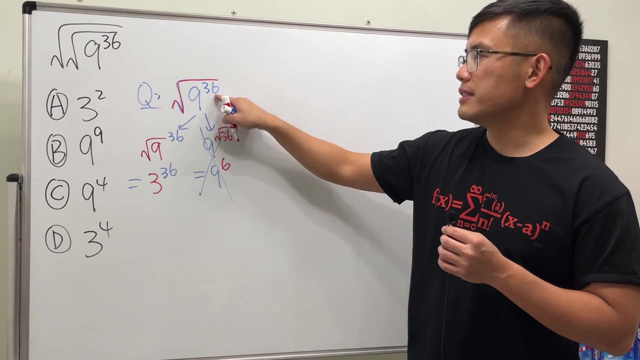 this is incorrect. This is okay. If you want to do the square root of the base, it's okay, And if you want to fix the power, you are not supposed to do a square root of the power. This is how, When we have a square root, and this is 9 to the 36th power, what we are going to get is the 9th. 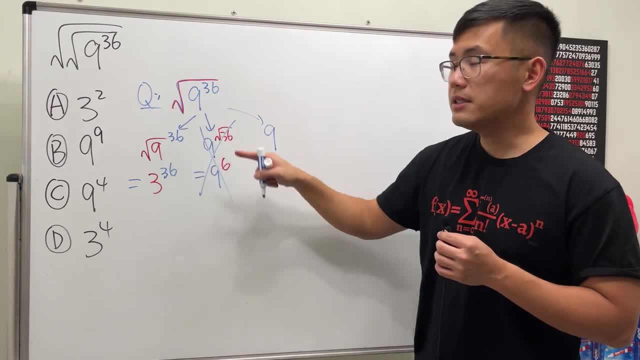 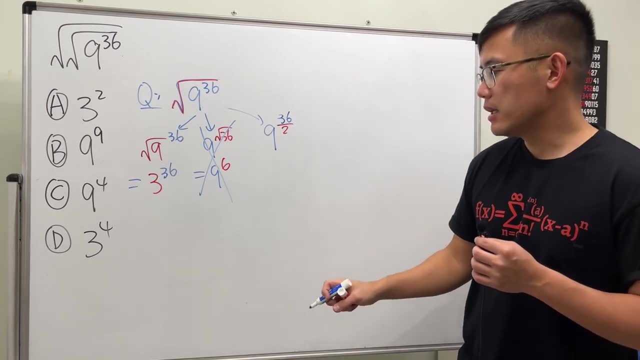 base. But instead of doing the square root of the 36th, we actually have 36 and then divide it by 2, right, Divide it by 2.. And the reason is because square root of x times square root of x is equal. 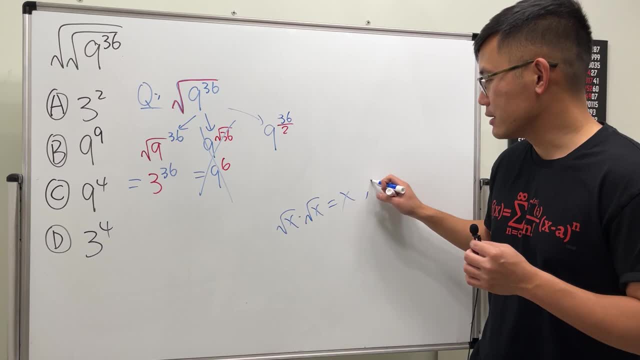 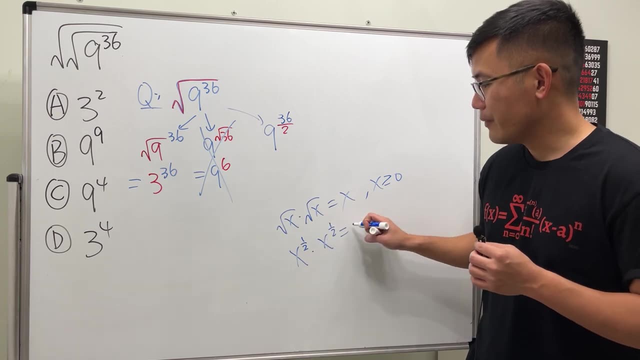 to x. yeah Well, assuming x is greater than or equal to 0.. And here you see, if we have x to the 1 half power times x to the 1 half power, this is equal to x to the 1 half plus 1 half is 1.. 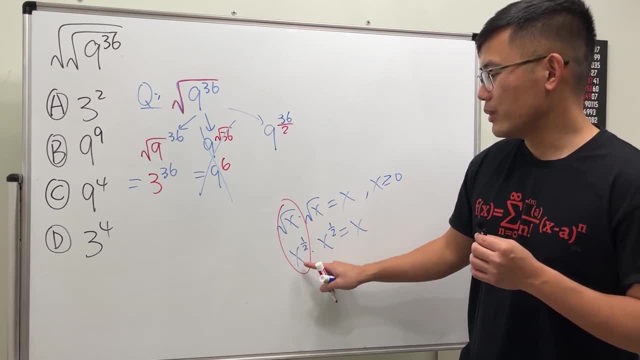 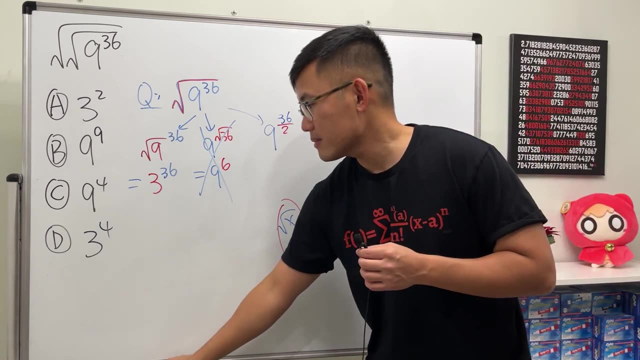 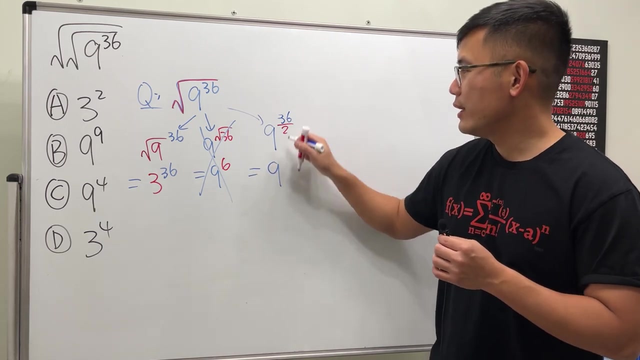 So the idea is that square root of x is equal to x to the 1 half power. So this right here is the half power and you multiply that with 36.. Therefore, if you want to fix the power, we will end up 9 raised to the 18th power And in fact this and that are the same thing.